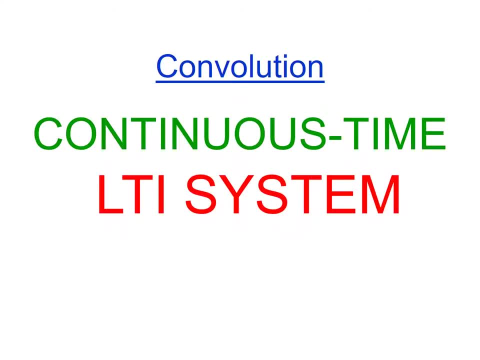 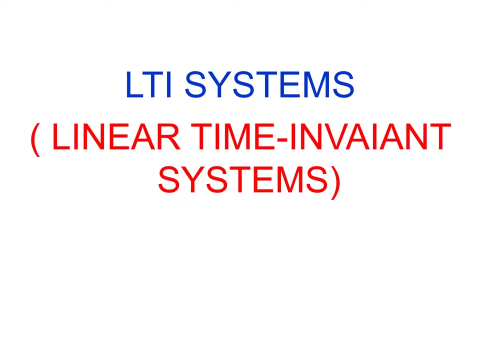 In this video we will learn about convolution of continuous time- LTI system. I would strongly recommend that before you view this video, you must view my video on discrete time convolution. Now, what is an LTI system? Just to repeat, LTI stands for Linear Time Invariant System. 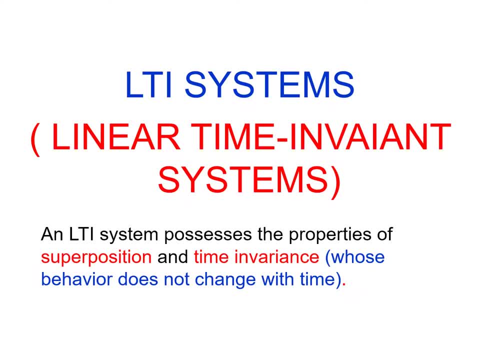 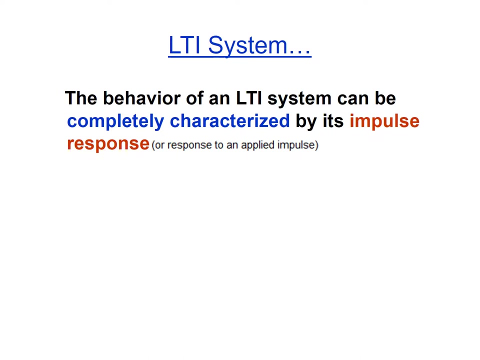 And an LTI system has two properties. Number one: it follows the superposition principle, that is, more than one signal can be applied one at a time, And it is time-invariant. That means it's time-invariant: Its behavior does not change with time. 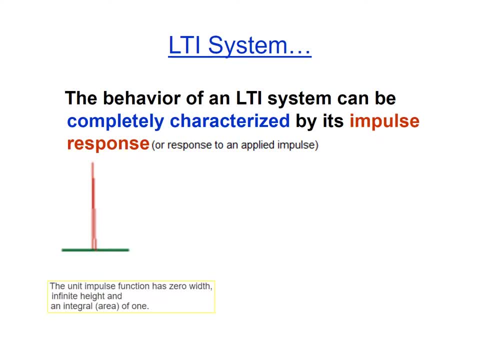 Now, any LTI system can be characterized by an impulse, Applying an impulse or a pulse of very narrow duration. So if this is an LTI system, we apply an impulse And we want to find its output. That output is known as the impulse response. 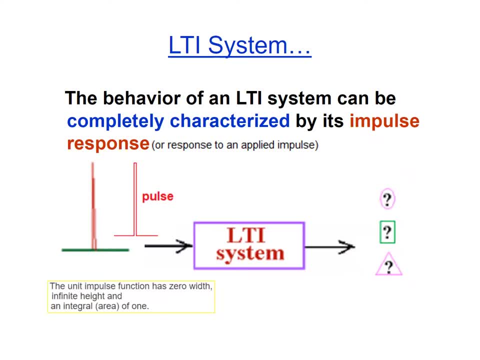 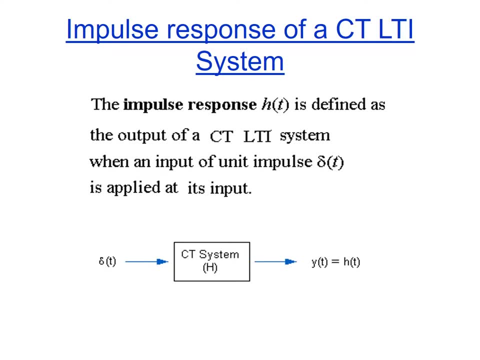 And in all our problem solving we use that impulse response. In case of a continuous time signal, the impulse response is represented by ht And the impulse signal itself is represented by ht, And the impulse signal itself is represented by delta t. So delta t is the input to the continuous time system. 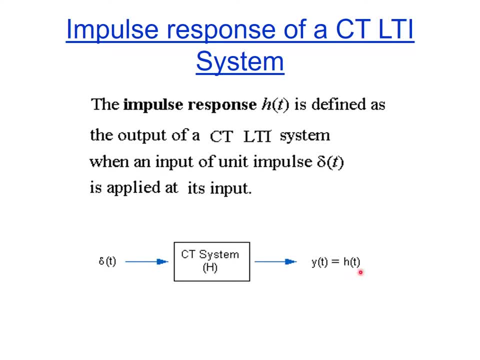 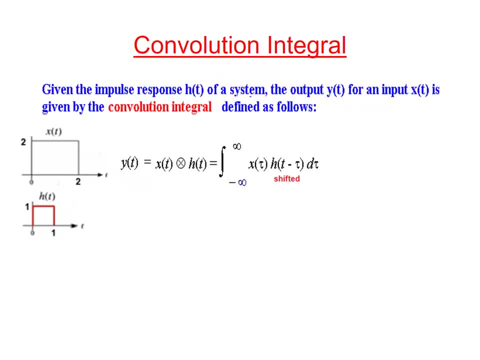 Then its output yt will be equal to the impulse response ht. Now the formula for convolution integral, or convolution integral itself, can be defined as It is the impulse response. It is the impulse response of a system: ht Multiplied by the input signal st. 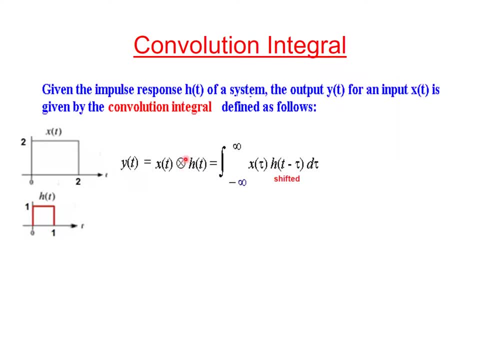 Sorry, not multiplied, but convolved. So this is the signal for convolution. So st convolution ht will give an output yt. So this is how we define convolution And actually the more practical form is That it is defined from integral minus infinity to plus infinity. 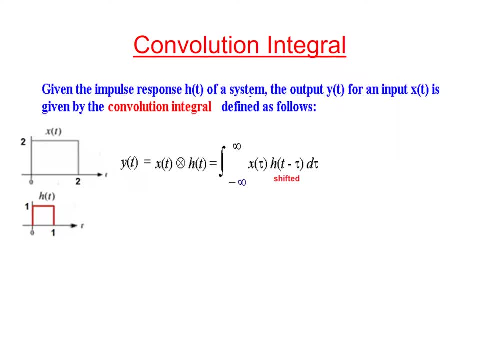 x of tau multiplied by ht minus tau, dt. Now ht minus tau is actually shifted function, Shifted from the origin. We will see with the practical example, And this diagram may give some Idea, what is convolution. So we have a signal: ht. 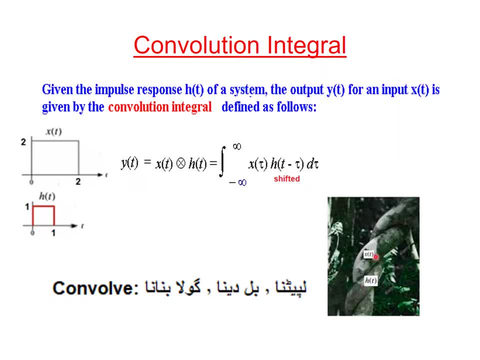 And we have the impulse response ht, And the combination of the two is the output yt Or the convolved output yt. There is another form of representing the same thing, That is, Instead of shifting h signal, We can shift x signal. 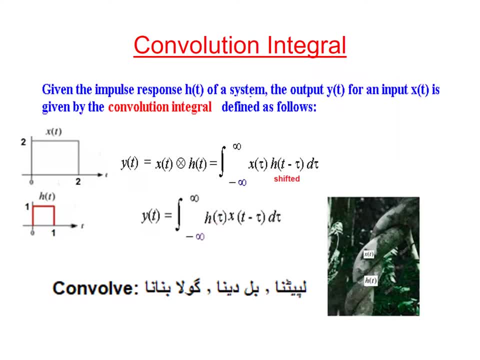 And h tau remains constant. So here ht, h tau was constant And ht minus tau is the shifted form. But we can get the same result By keeping h tau constant And shifting the signal input, signal x. These are some of the steps that we will be following. 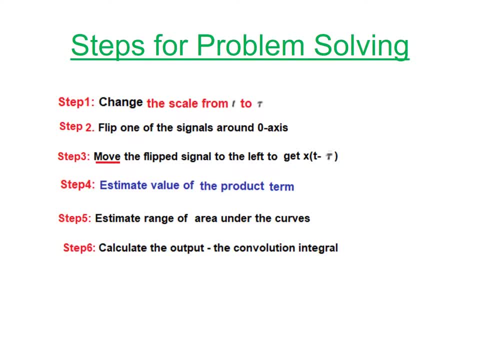 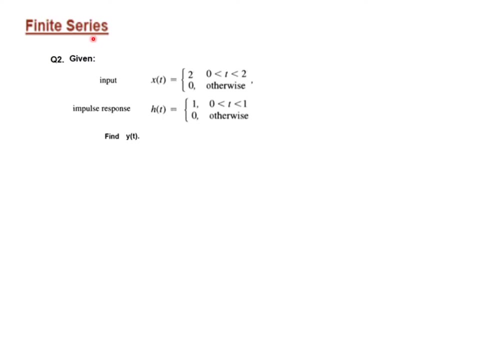 In solving the problems. I will not describe them now Because you will not be able to understand now, But when we go through an example, Then these steps will come And you will understand them. There could be two types of problems. It can deal with the finite series problem. 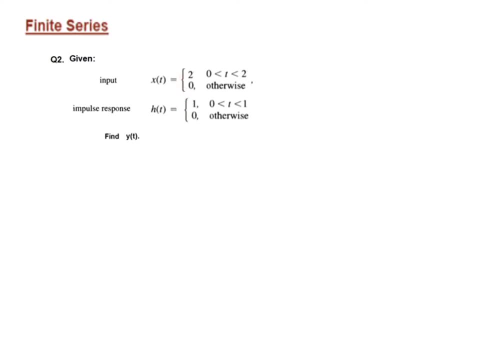 And infinite series. This is a finite series. example, We have a signal xt Given by this relation And also the impulse response ht Given by this relation, And we need to find the convolution yt. So the first thing we do, 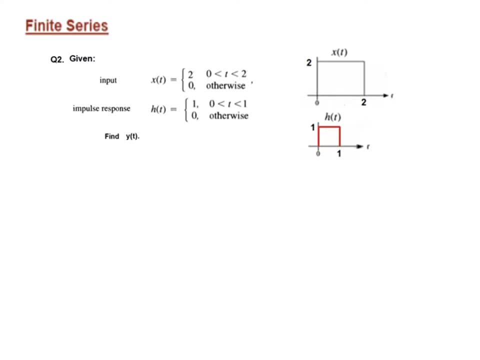 Is we draw the A2 signals. Now. note that xt is defined to be Having amplitude of 2.. So amplitude of 2.. And Its duration is from 0 to 2.. So from 0 to 2.. 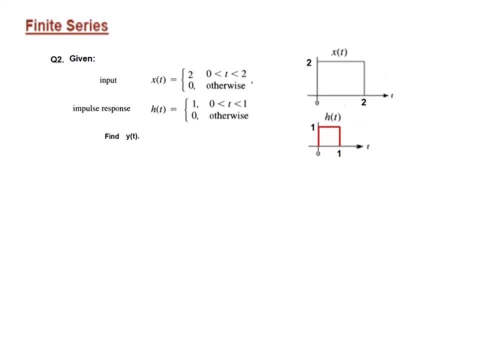 Its value is 2 constant. Similarly, xt has a value of 1 constant from 0 to 1.. So this is 1 from time 0 to 1.. So this is the pictorial form, And now we come to step number 1.. 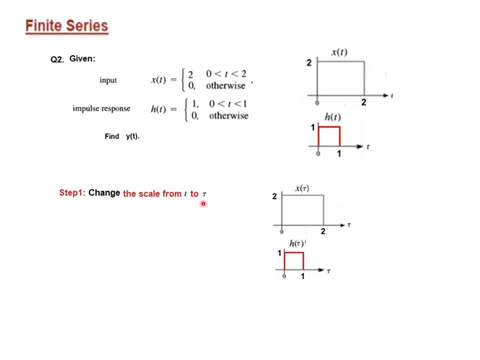 So the first step is To change the scale from t to tau, So everything t here will be changed to tau. So it is now x- tau And the time axis is tau. Similarly, h- tau And the time axis is tau. 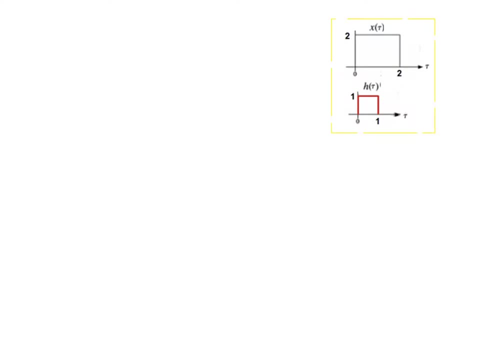 So that is the first step that we do. So this is what we got after changing the scale. Now we come to step number 2.. Flip one of the signals around x axis. Similarly, h signal is flipped, But, as we discussed earlier, 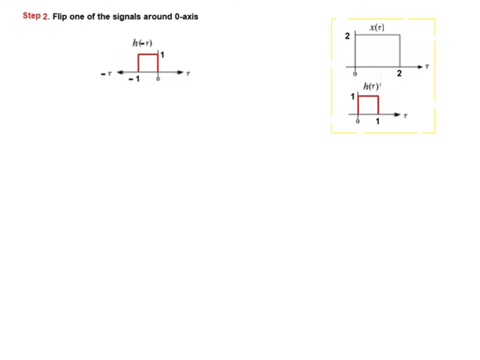 That x can also be flipped. So here we will flip h signal. So we just flip it around this 0 axis, Flip it like this, So this will become the inverted form, Or flipped form, And it will be now h minus tau. 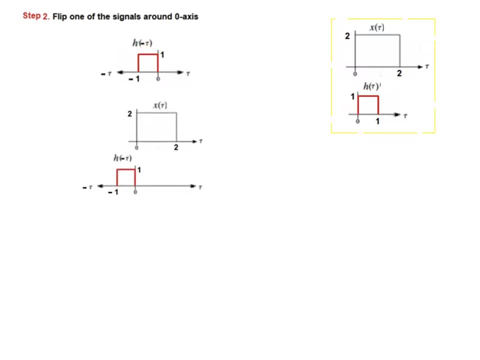 Okay, So the relation of two signals now becomes x, tau and h minus tau. The third step is That we move the flipped signal to the left To get x, t minus tau. So we are moving this towards left. So 0 will become t. 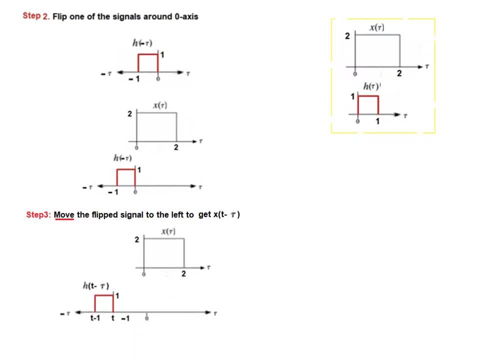 And so this will become t minus 1.. So this is now the relation between the two, The input signal And the flipped and shifted impulse. response For 0. It is now t And for minus 1.. We just add t with this. 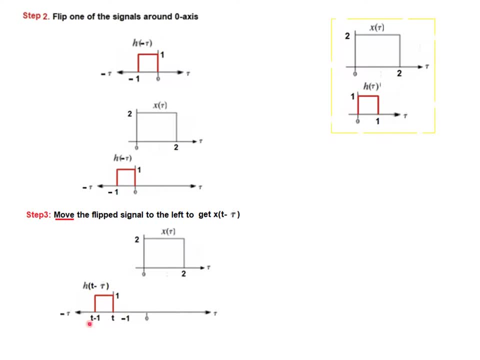 So it will become minus 1 plus t Or t minus 1.. Okay, You will be able to understand it in a better way If you just consider That this flipped signal has been mounted On a train trolley. So here is the t. 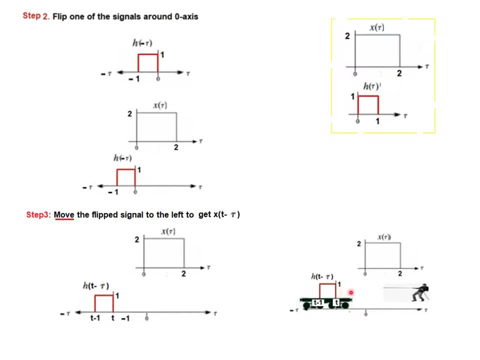 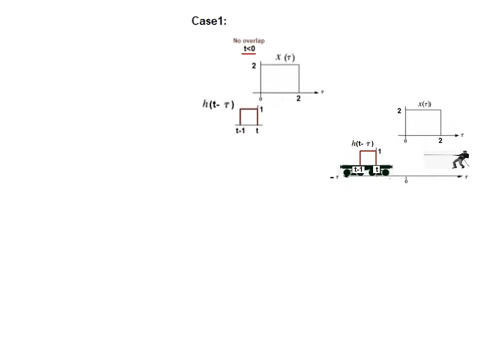 And this is t minus 1. And we will gradually pull the trolley along. Okay, So we are pulling it And let us stop here, Just short of 0.. So this is the- We will call it case number 1.. 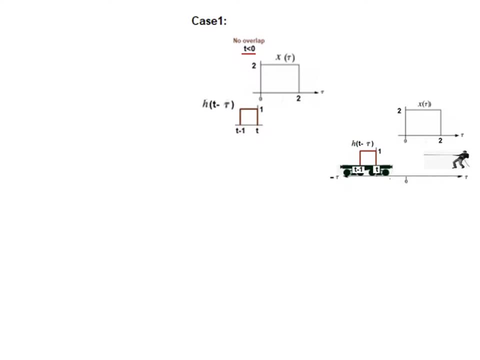 Where t, This t Or this t Is less than 0. So it is not 0. It is prior to 0.. Less than 0. Similarly, here, It is less than 0. So and. 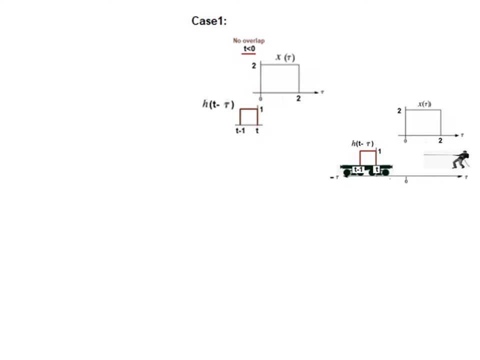 In this case. Now you can see That there is no overlap between the two. Two signals are not overlapping. Okay, Now We go to step number 4.. Estimate the value of the product terms. So if it was overlapping, 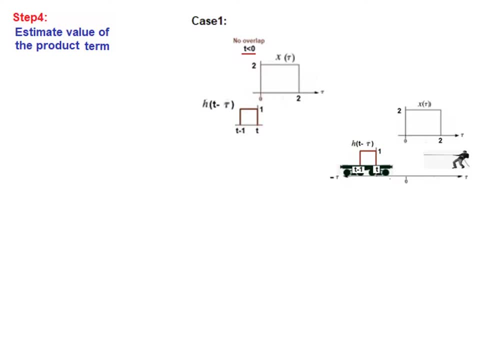 Then we could find the value of the product term, But since it is not overlapping, So there is no product term, And therefore x tau Multiplied by h t minus tau Will be written as. Will be written as 0.. 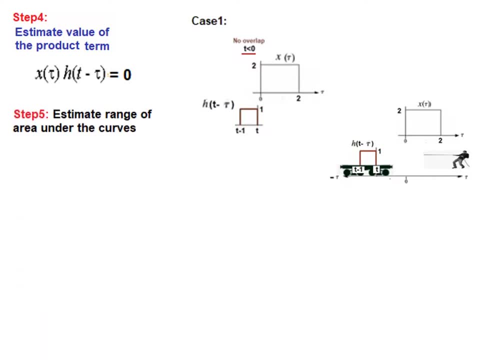 Because there is no overlap. We will now go to step number 5.. Estimate the range of the area under the curve Now, since there is no overlap. So there is no Area under the curve Combined, And so The 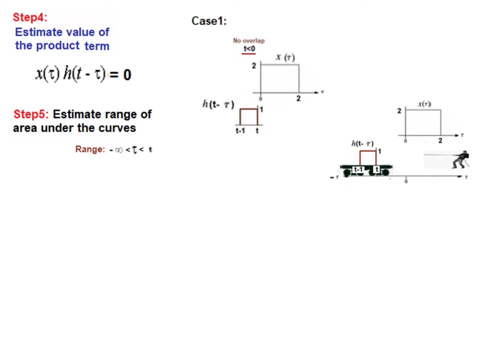 Range. We can say that It is from minus infinity to t, But there is No Overlap. Then comes step number 6.. This was the formula for the output, And now we will put the value of this multiplication, Which is 0, here. 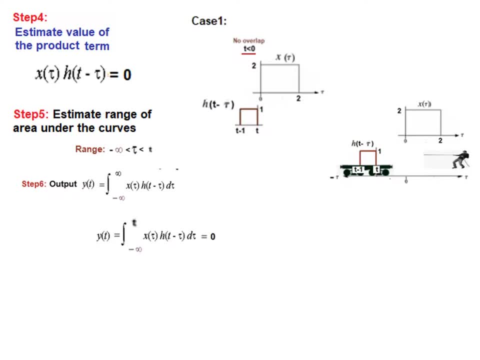 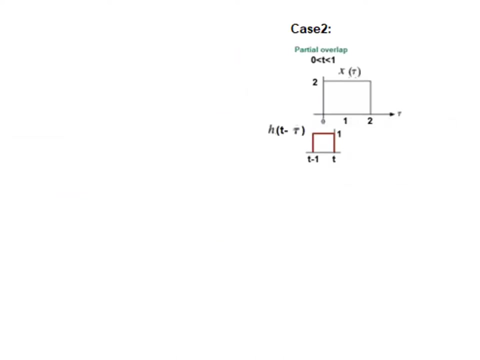 So the whole term or the output will become 0. And if you want to plot, We can plot it- That before t is equal to 0. The output is 0.. Okay, This is case number 1.. Now let's move to case number 2.. 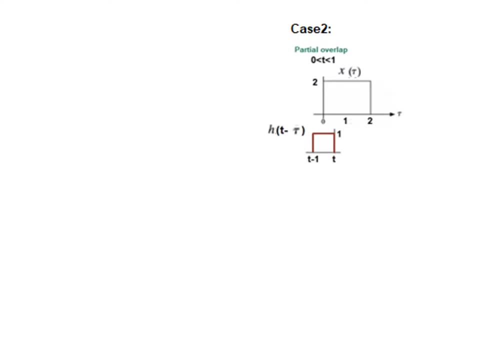 Where We have pulled the trolley further right And now note that t is between 0 and 1. So t is Between 0 and 1. And we have partial overlap. This portion is overlapping, So we can estimate the product. 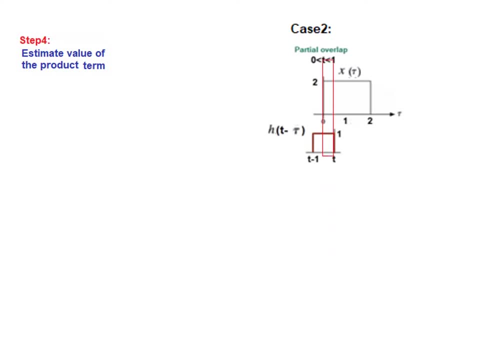 Okay, So this is the Overlapped portion And the product will be: X has a value 2. All the way, So here also it is 2. And this has value 1.. So the product will be 2 multiplied by 1.. 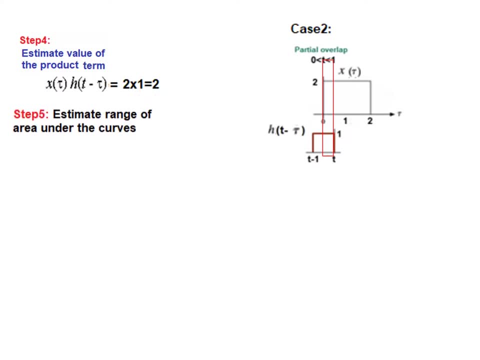 Is equal to 2.. This is step 4,, 5,, 6.. We will keep on repeating For every case. So estimate the range Of the area under the curve. Now We have to be very careful here. 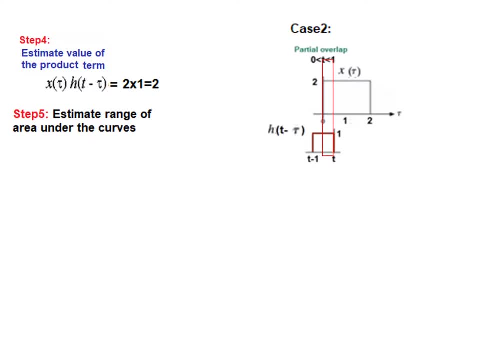 To find the range, Because that Determines the whole solution. Okay, So what is the range of this area? We don't know What is the starting point here, But we know this: This starting point is 0. So we will take that as. 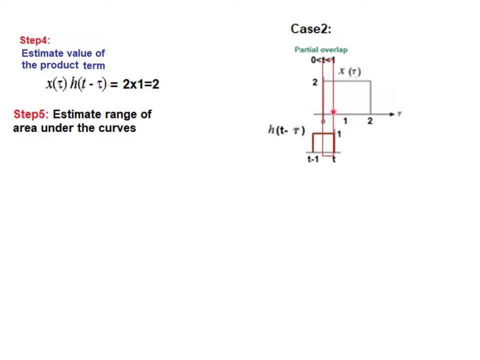 Starting point And we don't know What is the ending point here. So we will take this As the ending point, Which is t. So our range is from 0 to t. So tau Is between 0 and t. 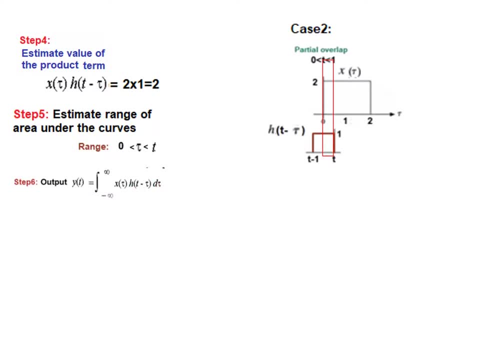 And then We go to step number 6. We put in the formula Now: This multiplication Is equal to 2.. So Instead of this We write now: 2d tau Integral. We put the range Instead of 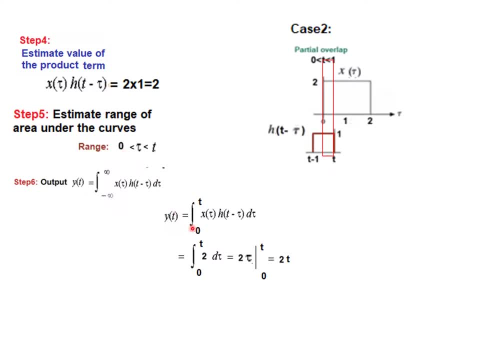 Minus infinity And infinity. Now We put the two range 0 and t, So If you integrate It will become 2 tau And the limits 0 and t, And so The answer is 2t. 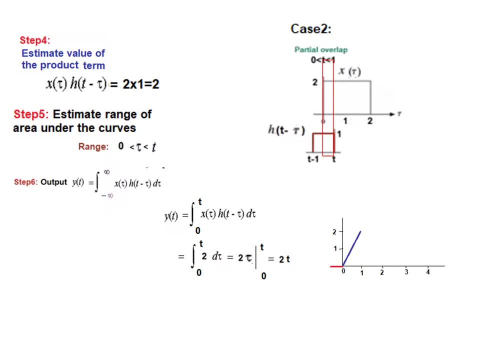 And We can now plot it Slope Of Slope Of Value 2.. So 2t Ramp Function, Okay. Now The third case Is the moment This t Crosses. 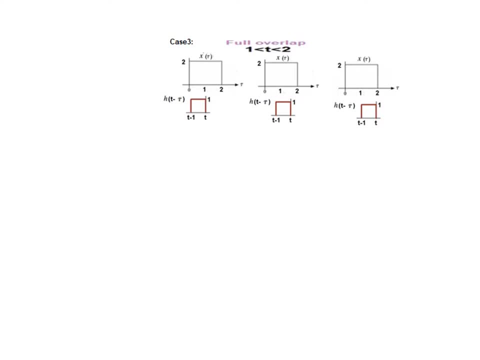 1., Then Just Add 1.. It is now Fully Overlapped. Then Even 1. Crosses 1., Then Just 2.. Then, Even If You Move, 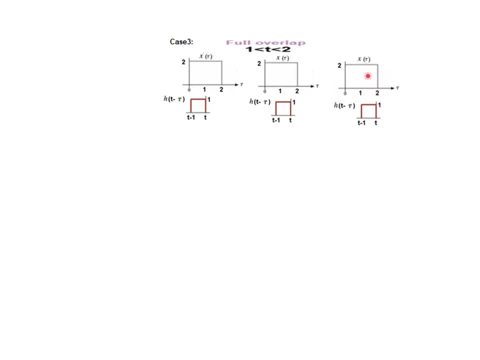 Further. It Is Still Fully Overlapped, And Still Move Further Short Of 2. It Is Still Overlapping. So Our Overlapping Range Is Now: 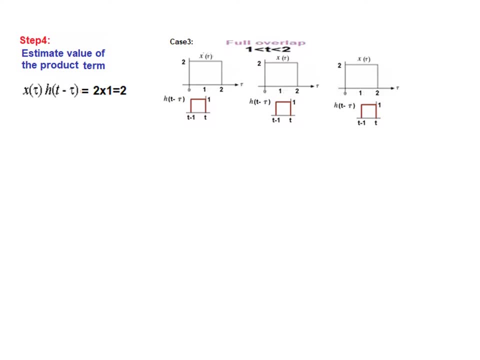 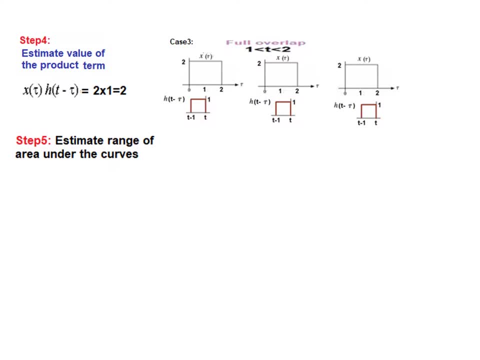 2. Here. 1. Here, So All. 3. The Other End Which We Can Now In All The 3. Cases In The Same Range, Minus: 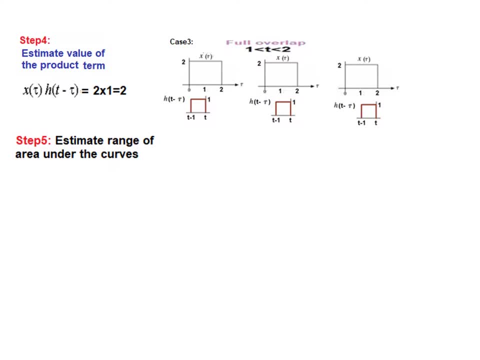 T, 1. 2. T, Both Are Very Distinct, Known Clear, And So Point. Similarly. We Don't Know What Is The Point Here. Neither We. 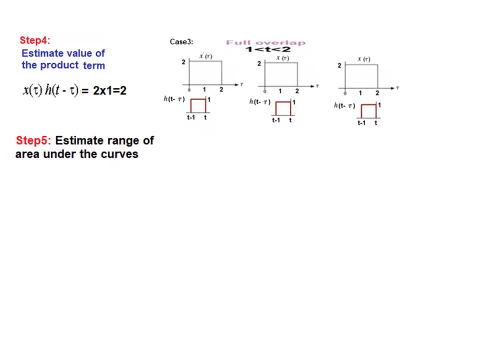 Know This Point, So And Same Here. That Is Why These Two Are Very, Very Clear. Therefore, And Then Putting In The Values And The Formula. 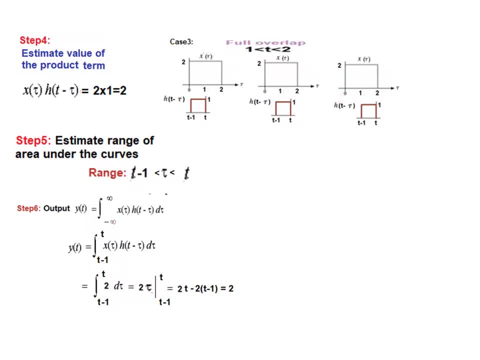 Same Value: 2., 2. Into 1., 2. Into 1., 2. Into 1.. So 2., 2. D T. But Now The Value. 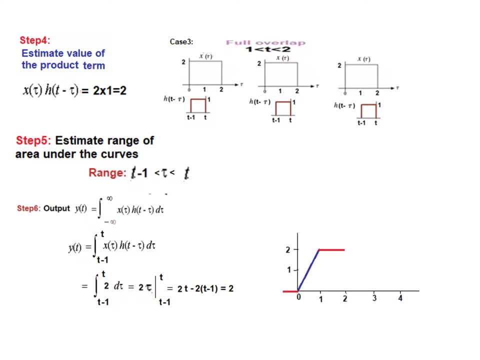 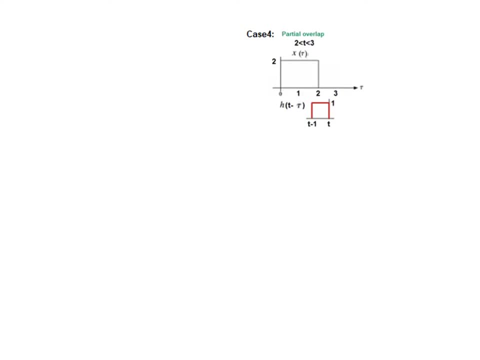 So Let's Go To The Graph. So From 1. To 2. It Is A Straight Line Of Value 2.. Okay, Now We Come To. 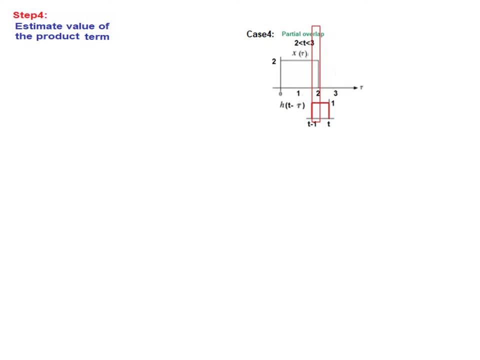 Case Number 4.. Where T Will Overlap. You Can See There Is A Partial Overlap Only, And Now We Will Estimate The Product Term. 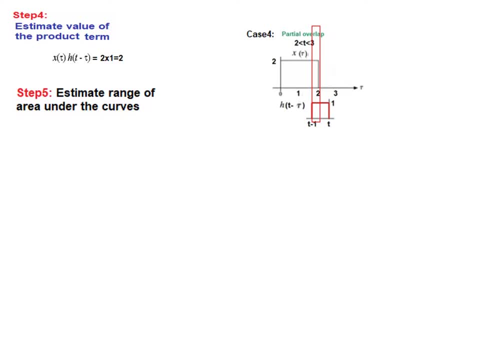 Again, Even In The Partial Range, It Is Multiplication Of 2. The Range, And Now We Have To Find Out What Is The End Point. 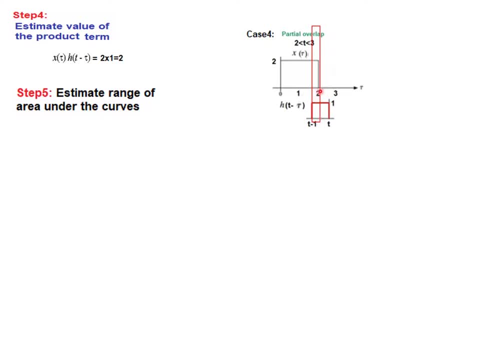 And What Is The Start Point? Now, The Start Point Cannot Be Found From Here And Then Just Put In The Formula, The Values, So To